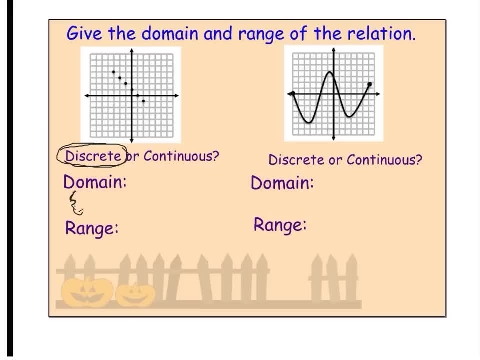 Kind of hard for me to write on my iPad These curvy or like really cute little brackets to indicate the domain and range the numbers that go inside. So remember, domain is like your x's, So really it's just asking what are all the x values that we see in the graph? 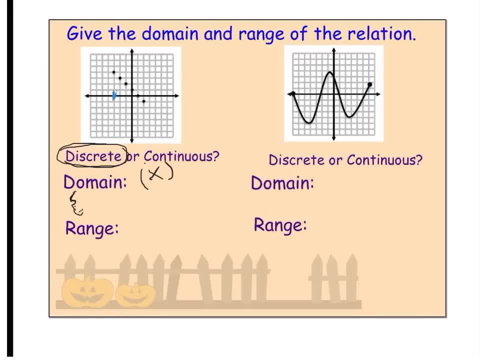 So if I look at this first point here, what's the x value there? Well, that first x value there is going to be negative 3. And I would just keep doing it for the next point. So the next point here, that is negative 2.. 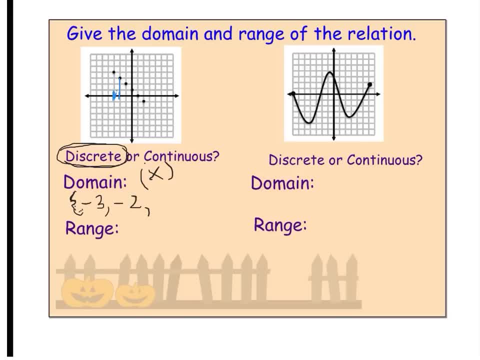 And then I would keep doing that. So negative 2, negative 2.. Negative 1.. And I also have 0,, 1, and 2. And then I would close it. And now my range: well, that's just the corresponding y values that go with my x values. 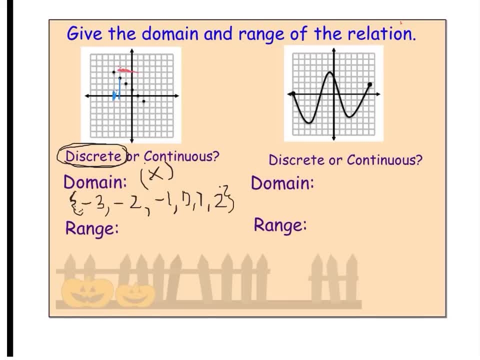 So if I start here, what's the y value for that point? Well, open up my bracket here. The y value there is 4.. My y value here is 3.. And I go ahead and I write the y value. So 2,, 1,, 0, and negative 1.. 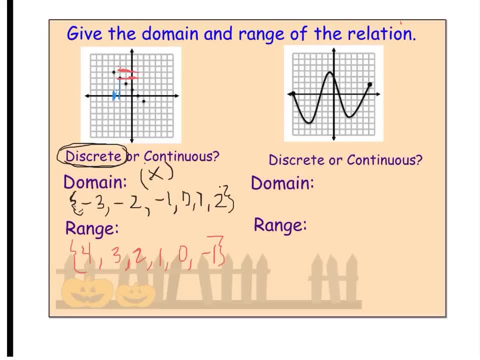 That is my domain and range. here It's just the x values and just the y values. Let's look at the graph on the right. So this one is a continuous graph, And I know it's continuous because I see that there's a curve going through. 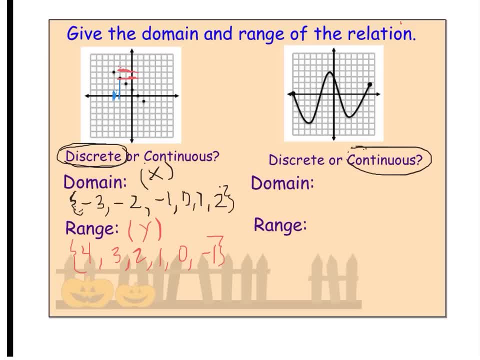 that connects all the points that are really there. So, talking about domain and range, when we have a continuous graph, we generally write: We write it as an inequality. That's just the fastest way to do it. So the easiest way to do it is if we're thinking domain. 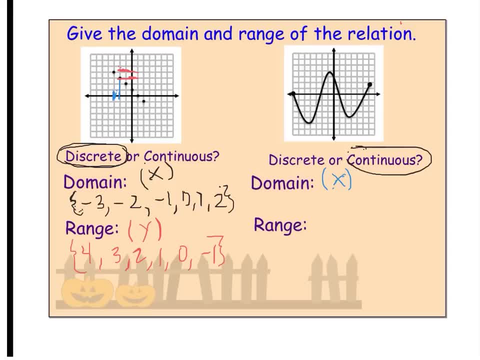 So I'm talking about x's. If it's a continuous graph, the easiest thing to do is to find the smallest x value, So that's here, And the biggest x value, which is here. That is going to set the boundaries for our inequality. 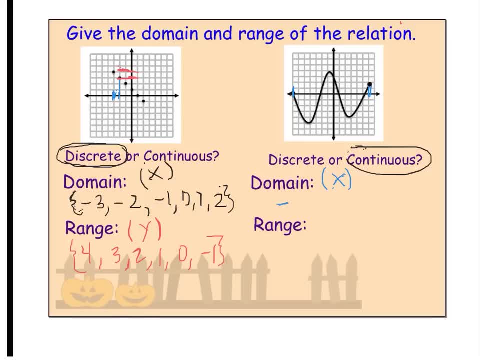 So our smallest x value is negative 7.. Okay, Oops, let's try to write that a little neater there. So that is negative 7.. Sorry, it's being a little finicky with me, So negative 7.. And we also know the max is going to be 6.. 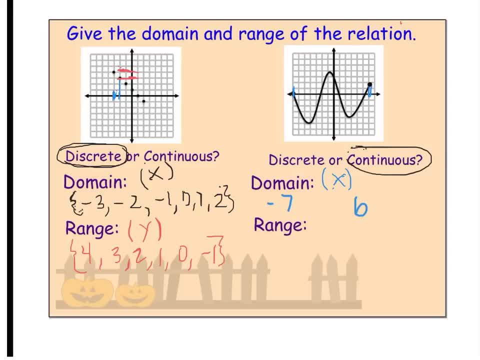 So then I just have to figure out what goes in here. Well, I know that this is almost like kind of an and component inequality, where the graph is between those two, So I can write it as: less than or equal to x is less than or equal to 6.. 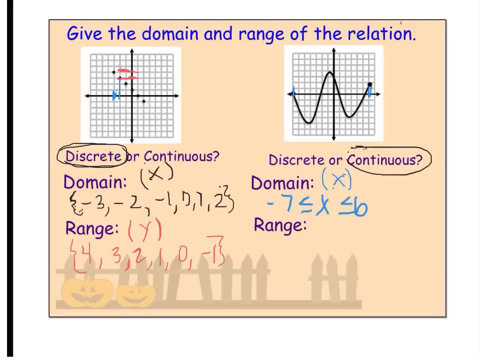 And that would be my final answer there. So I have all these x values, anywhere from negative 7 up to 6 are my possible x values. I want to look at y. I have my max y there and my minimum y, So now it's the lowest one. 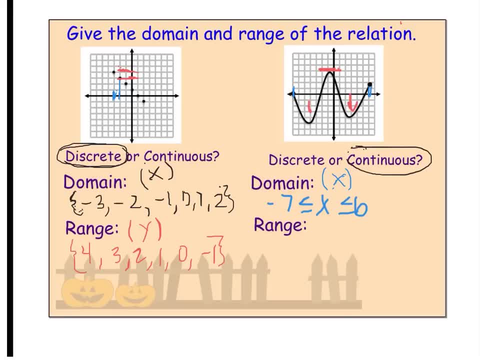 So notice I have a low point in my graph here and here, But this is the lowest point, So I go with that. So then my range would be: Come negative. 5 is less than or equal to y, Because I'm talking about y. 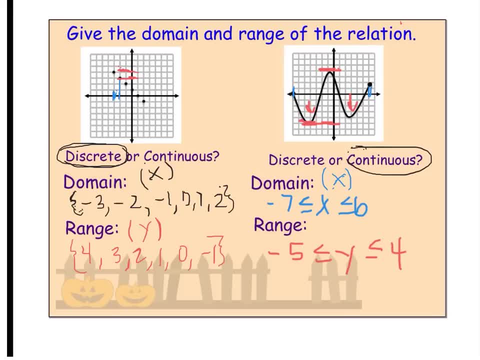 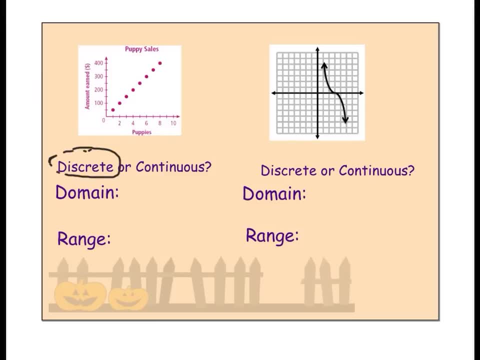 Which is less than or equal to 4.. And that is my inequality for my range. Alright, my next graph I can see is just points. It's got to be discrete. Let's talk about our domain. We're going to use those brackets. 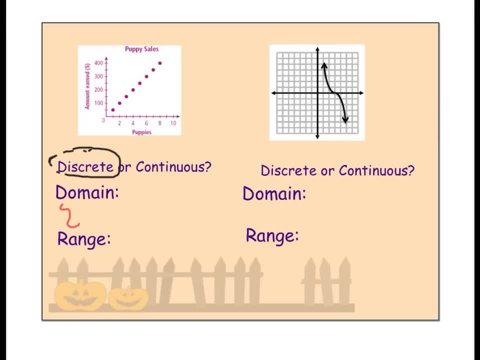 We're talking about our x values here And now. if you get tired of listing these out, because we have kind of a lot, you can actually list the first couple. So, like I can see, I have an x value of 1.. 1,, 2,, 3.. 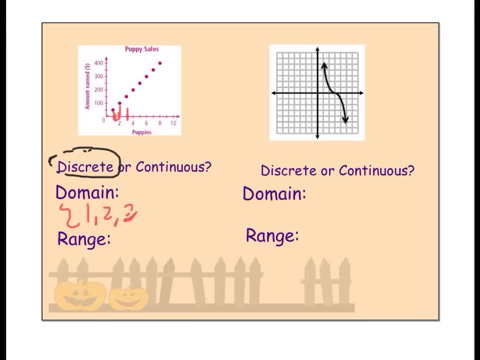 It's going up by 1's. You can actually use shorthand, So put your 3 and then do dot, dot, dot And then put your max, which is 9.. Do the same with my y's. So my range, my minimum, is going to be 50.. 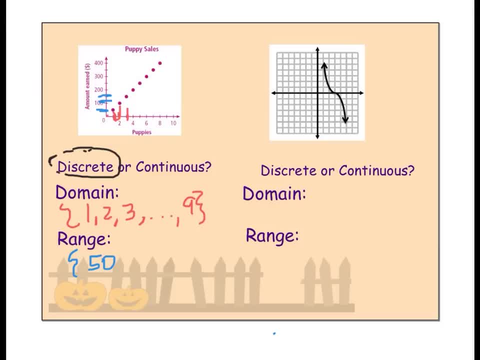 And I notice I'm going up by 50's because I'm at 100 and then 150. And then I can do dot, dot, And then my max is going to be 400. And then close my brackets. Okay, moving on to the right. 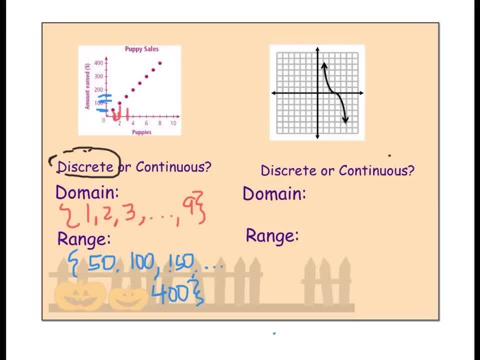 I see it's a line, It's connected, It's curvy, It's got to be continuous. Now let's talk about the domain. here You guys might notice there's some arrows right. There's an arrow there And there's an arrow there. 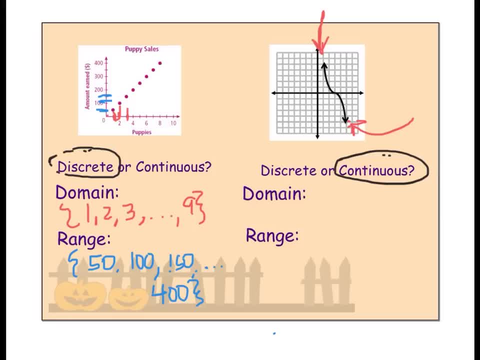 What that tells me is that the graph is actually going 2.. 2, infinity this way And negative infinity this way, And I don't have any boundaries on my graph, So it looks like I actually can use any x values going left or right. 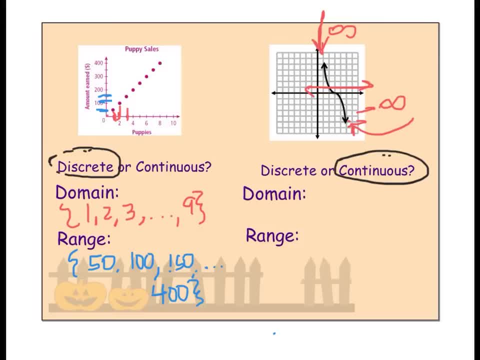 If I extended my graph I would see that more x values are used, the bigger the graph gets. So for domain you could say all real numbers, So a r, n, Or maybe you'll say negative infinity, Less than or equal to x. 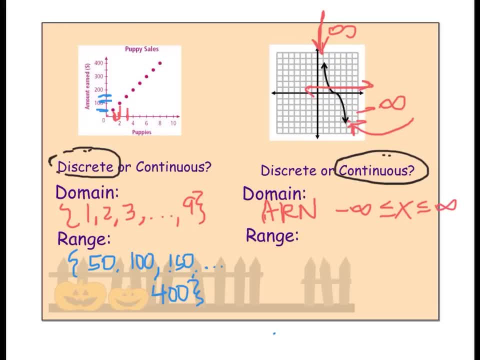 Less than or equal to infinity. Now the range is the same thing. These arrows here tell me I go to positive infinity in the y direction and negative infinity in the negative y direction, Or, if you like, all real numbers. you can do that. 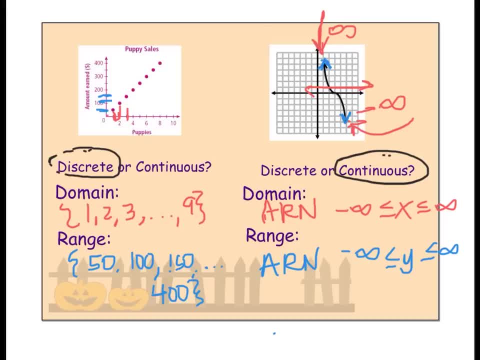 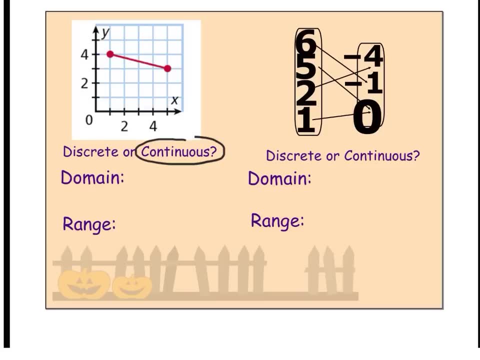 So we watch for all real numbers when we see arrows on our graph. All right, another graph. It's a line. It's not curvy, But it is a line, so it's got to be continuous. My domain is my x's. 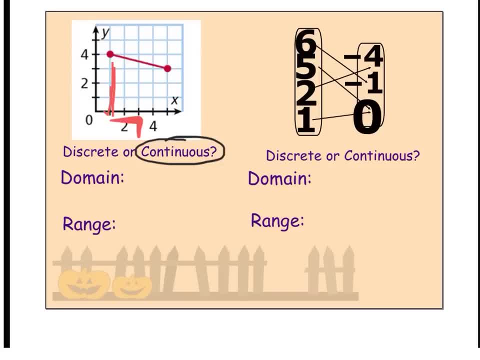 So here's my minimum: x is 1.. Oops, My minimum should have been 1.. And then my maximum is going to be 5.. So I'm going to write it as an inequality. So 1 is less than or equal to x. 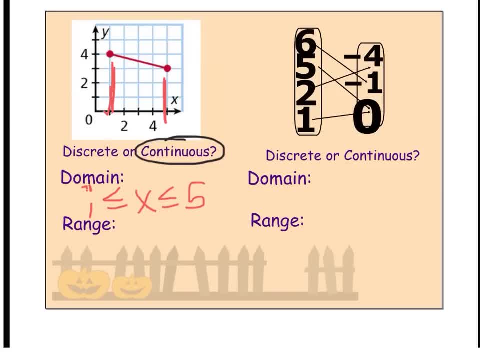 Less than or equal to 5.. Do the same thing for my y's. Y is my minimum, y, which is here, And my maximum, So 3 and 4.. So 3 is less than or equal to y, Less than or equal to 4.. 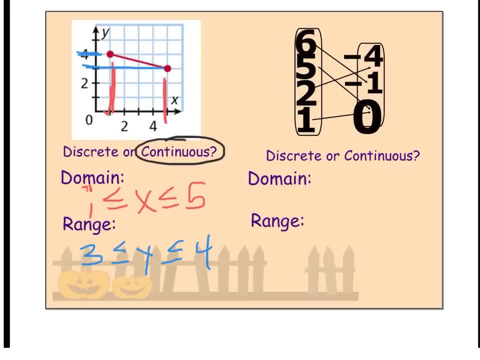 And that's always my general setup for a continuous graph. We can actually tell, or at least get a good idea, if something is discrete or continuous from a mapping diagram. Now, since a mapping diagram is used here and that's our usual x and y,